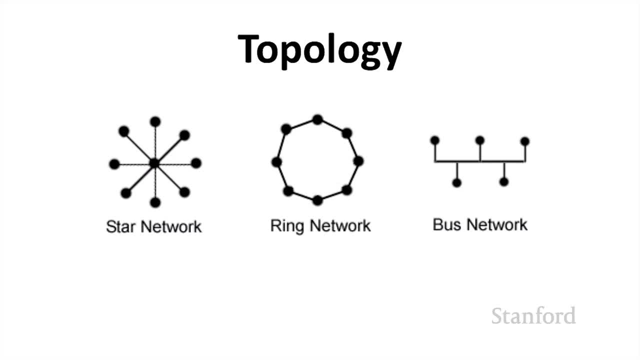 and they're all on the internet, And somewhere in that room or in a nearby room is the Wi-Fi router, And so all the computers talk to that individual, And if the individual Wi-Fi router goes down, nobody can talk to each other. 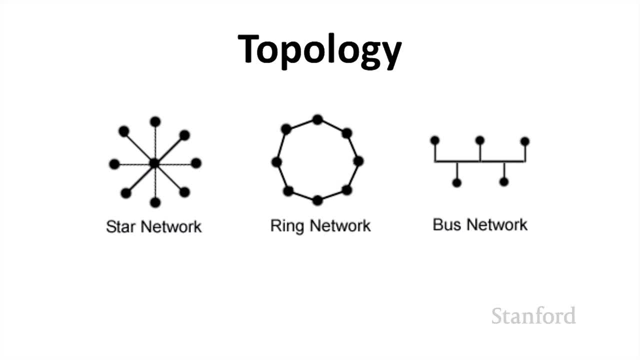 So that's a star network, A ring network. as you can see, here we have a bunch of computers And they're all hooked with, one following the next, following the next, following the next, And so depending upon how many nodes you have, 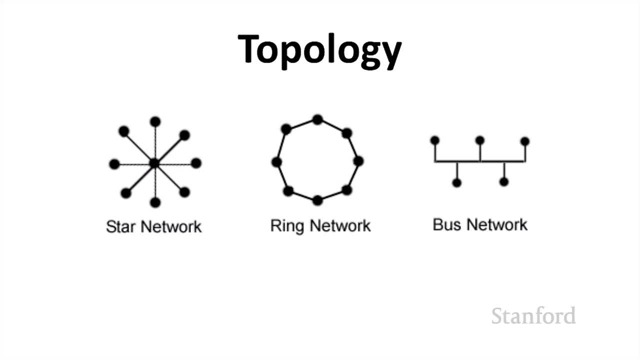 this actually takes less connection medium than our star network does. Ring networks are commonly used, for example with optical cables. One of the problems with a ring network is that it's not a common network. One of the problems with a ring network at least. 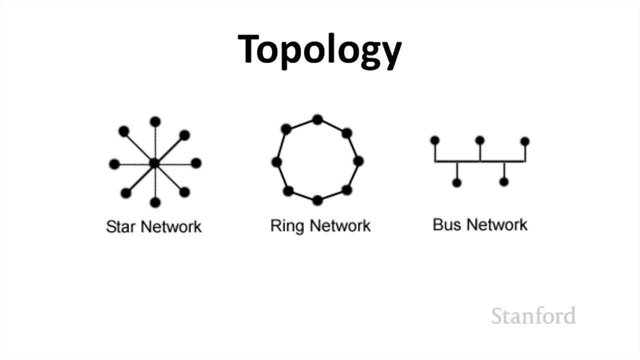 as the way they typically work is, if one of the nodes goes down, this message has stopped traveling around the ring. You can certainly imagine having a ring where, if one of the nodes went down, the message has started going in the opposite direction. 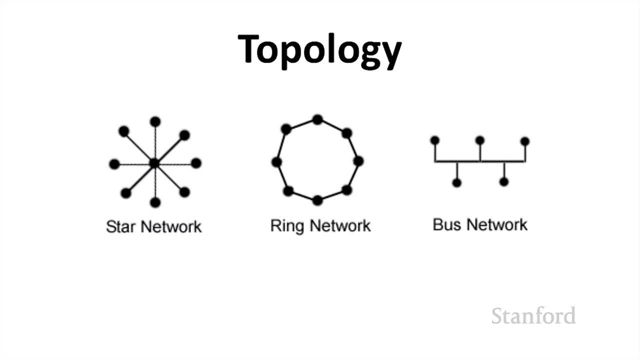 But that's not typically how they work. And then, finally, our last example here is a bus network, And in a bus network all the computers are connected to a common cable. This sort of network used to be quite common, connecting computers together. 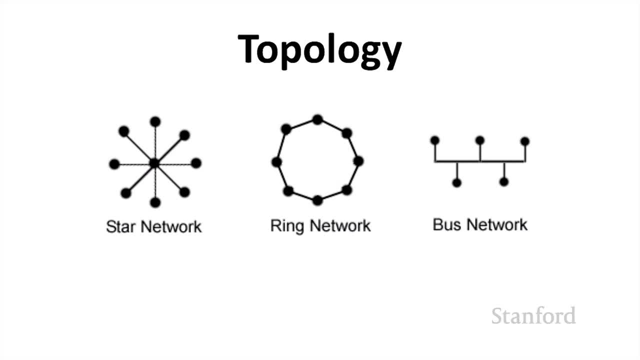 They're in a classroom. Bus networks also have their own set of problems, And, in fact, each of these networks is going to have to have different rules for how they govern and how they work, And so one of the problems with the bus network- 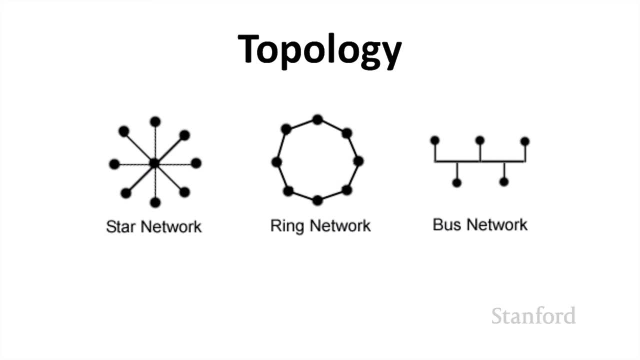 is if multiple computers on the network try to send out a signal at the same time, you have a problem where there's contention on the line And the network needs to have rules for what happens when two computers are simultaneously trying to use that bus. 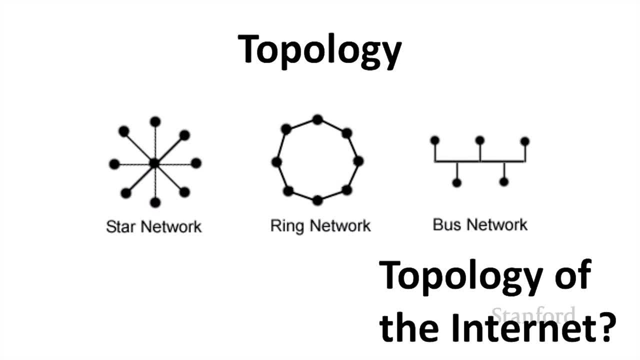 So one question we can ask ourselves is: what kind of? so we've seen three different types of networks Here. what kind of network is the internet? And that actually turns out to be a trip question, because the internet is not a single network. 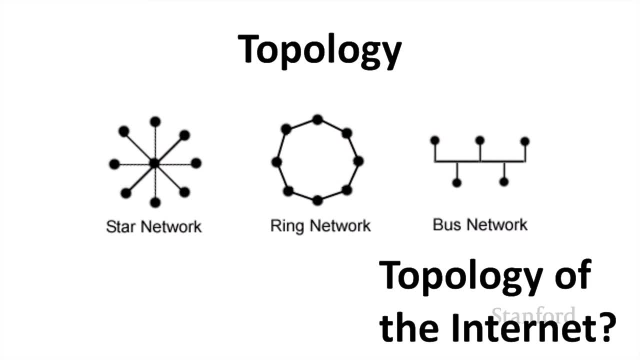 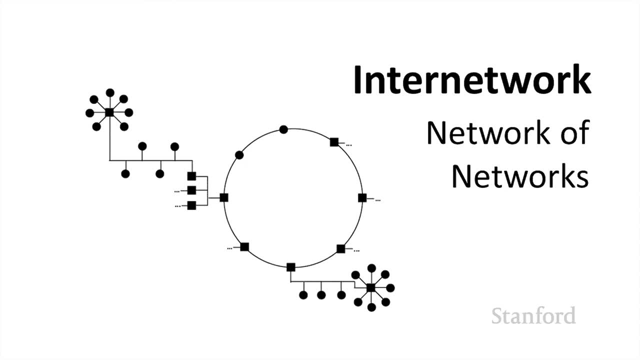 It is actually a network composed of different networks, And this is what we refer to as an internetwork, And so here I've got a drawing of a network of networks. This is the sort of thing that might connect different people on campus, So we might have a set of optical fiber cables connected. 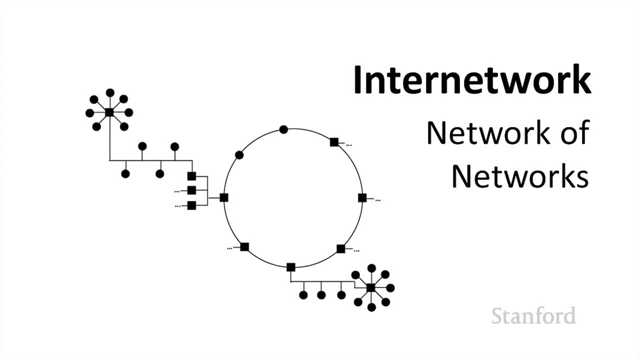 This is connecting the different buildings in the university, And so we've got like a ring connecting each of those, And then we might go from there to a bus network connecting different floors on a particular building, And then those individual floors might have their own bus networks. 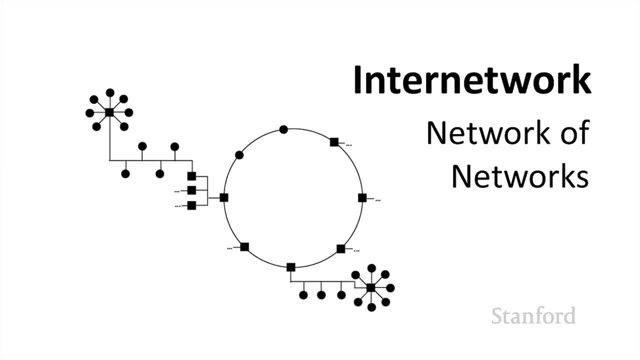 So we have a bus network, connect to a bus network And ultimately, for convenience, somewhere on that bus network we need to have our Wi-Fi router, And then we have different people connected into the Wi-Fi router. So this is just a small example of an internetwork. 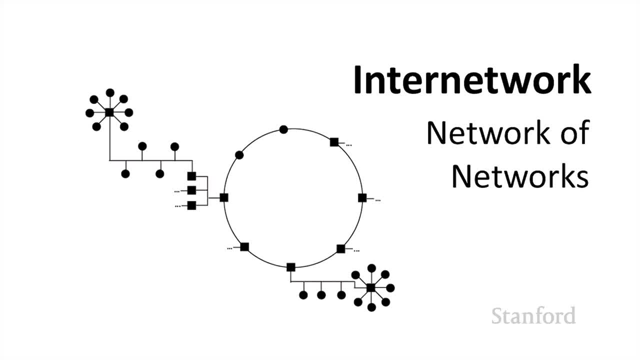 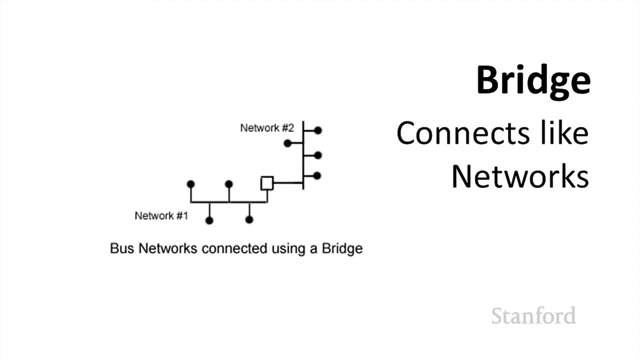 But in fact, the internet itself is composed like this, with different networks connected to different networks connected to different networks. Now there's different types of hardware you may run into when we're working with our internetworks, And so one of the devices is a bridge. 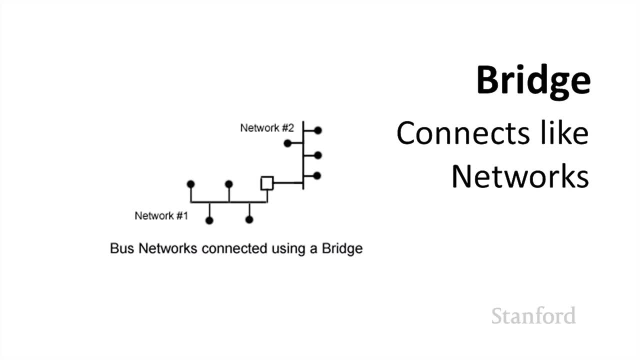 And a bridge is used to connect two different networks that are of the same type. So you can imagine, This is simpler than connecting different networks of different types. And so say, we have one bus network that's running across all the dorms in a particular complex. 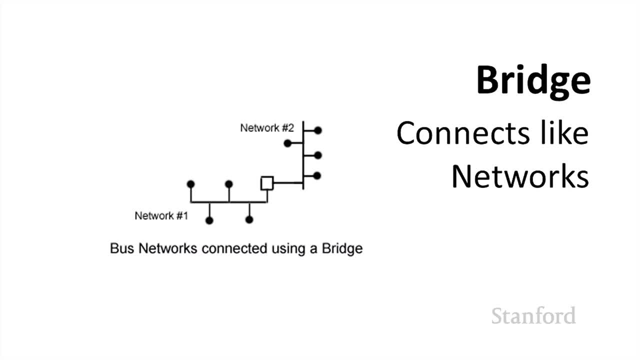 So say, we have a bus connecting all the dorms in Stern or all the dorms in FOMO, And then each of the individual houses might have their own network, And so we would need a bridge to connect one of those networks to the other network. 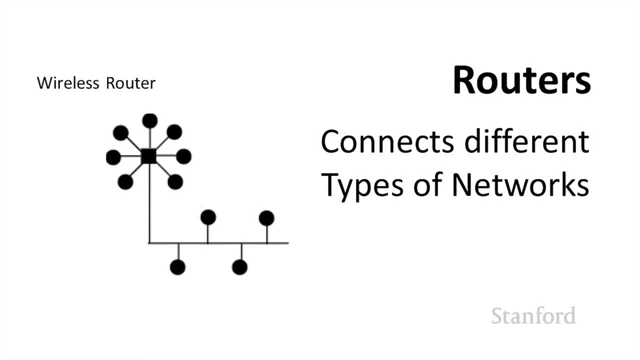 If we have two different types of networks connected together, we need a fancier piece of equipment, And so a router connects two different types of networks. This is probably most famous for wireless router. So if you hear people talk about wireless router, 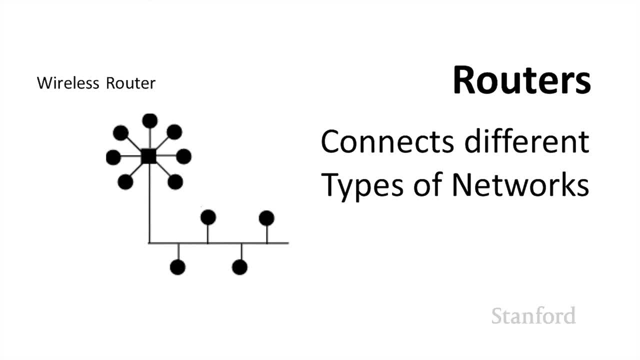 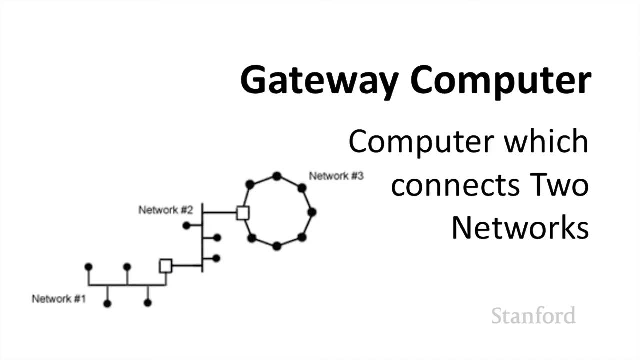 that is, a device that connects the wireless network, the Wi-Fi network, to some other type of network. You may also hear the term gateway or gateway computer. A gateway computer is a computer that basically acts similar to a router or a bridge. It connects different. 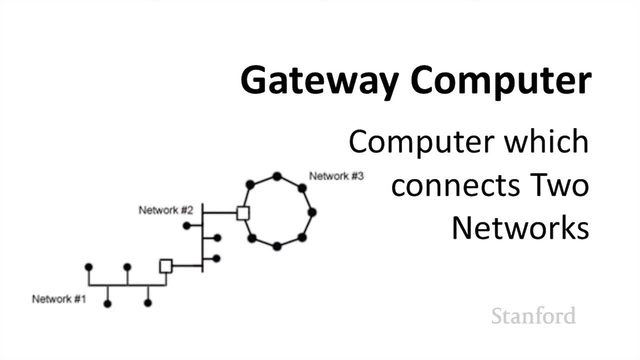 Networks together, The difference being that the router, or the bridge, is a very special purpose box that that's its only purpose in life is handling these messages, Whereas a gateway computer is a general purpose computer that, among other things, handles network traffic. Now we're not going to talk too much about the different. 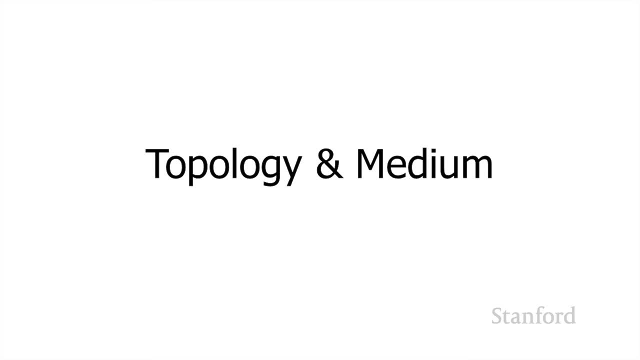 mediums that are available to connect our computers together. There's a wide range, ranging from plain old telephone service or POTS, which is the traditional copper cables used for telephone services, ranging up to cable networks, to fiber optic cables, to Wi-Fi, to satellite. 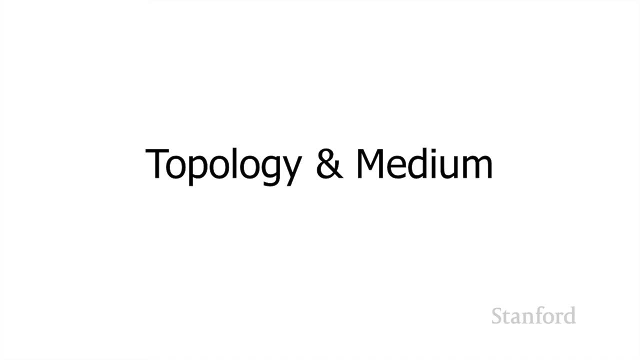 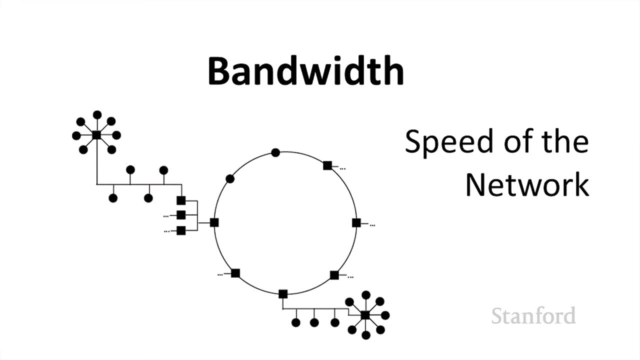 These all are different mediums, And there are different ways we can connect the computers in our network. One of the issues that comes up, though, when we're talking about different mediums, is the bandwidth, And so what the bandwidth is, what the bandwidth originally? 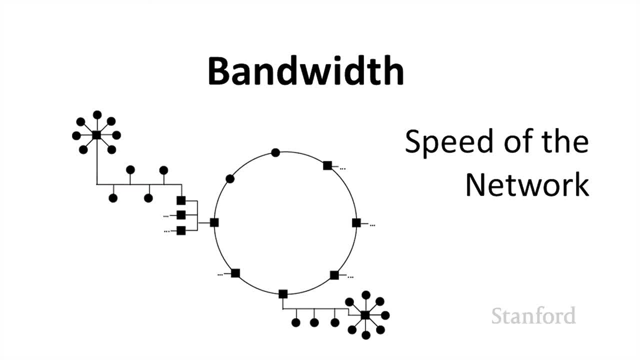 referred to, I suppose technically still does, although computer scientists tend not to talk about it this way. It is the band of frequency that set aside for that particular communication to take place. So the wider the frequency band we have available, the more messages we can send through. 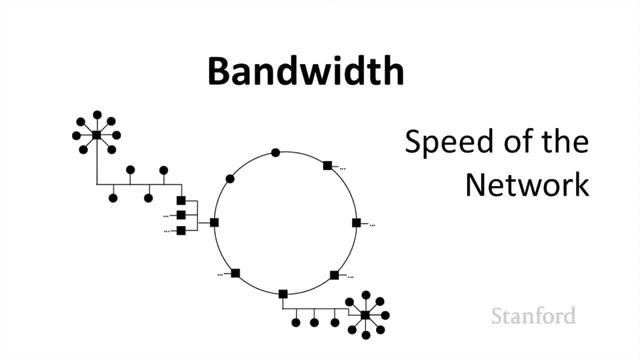 Computer scientists and generally. colloquially, most people refer to bandwidth as just the speed of the network. So if I have a lot of bandwidth that means I can send a lot of information quickly. If I don't have a lot of bandwidth, 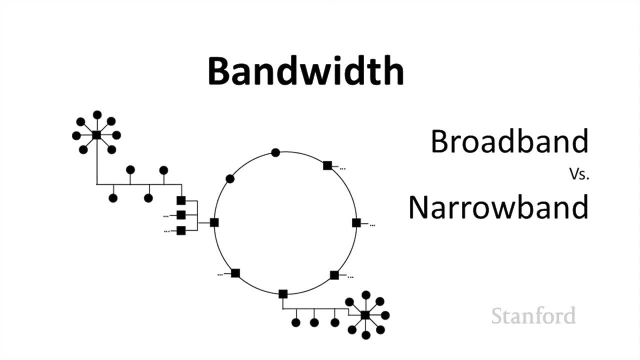 then I can't send messages very quickly. You may also hear the terms broadband and narrowband. Narrowband basically is plain old telephone line And plain old telephone service, or POT as it's technically referred to. I actually think it's kind of a cute name, POT that has very low bandwidth. 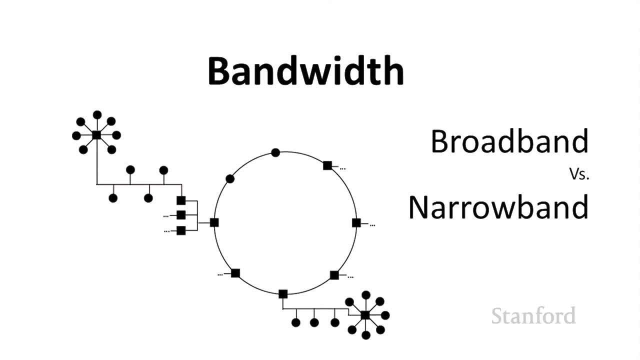 And we can't send much information through it And in fact, as we saw in one of our previous videos, if we want to send a five minute CD, it's going to take a lot of time. If we send a CD song over POT, it's. 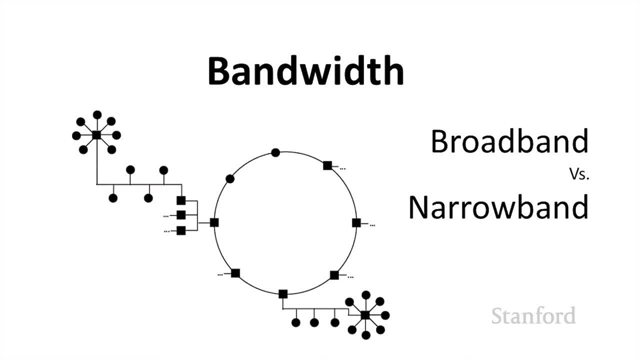 going to take about five hours, So that's pretty bad. The term that you'll hear more frequently is broadband, And this just refers to something that's not narrowband. Generally, these terms aren't in widespread use anymore, except for there's a fair number of companies that 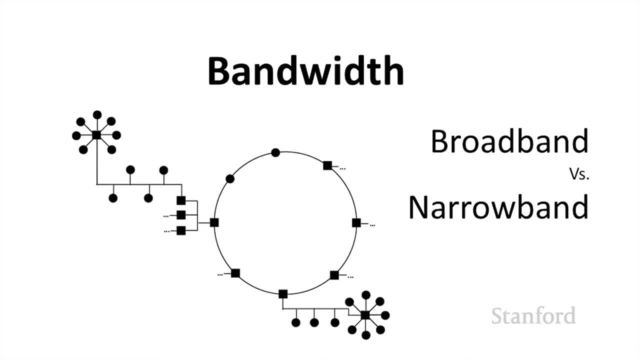 have the name broadband in them, because it used to be really cool to be broadband instead of narrowband, but now everybody's broadband. So you will still hear the term broadband banding around, mostly in the names of various companies that are out there. 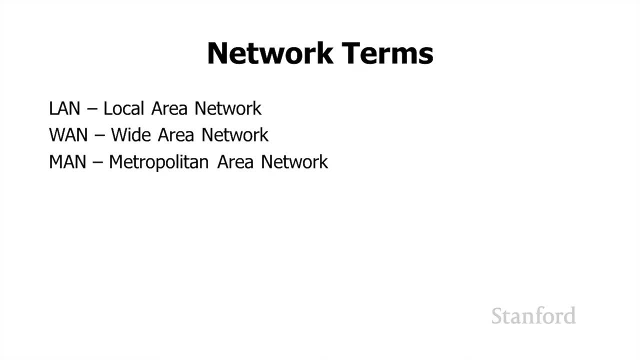 But that's what they're referring to. Here's some more terms you might run into. LAN stands for local area network. That's a small network. So if we have a classroom we have a bunch of computers hooked together in that classroom. we might have a LAN. 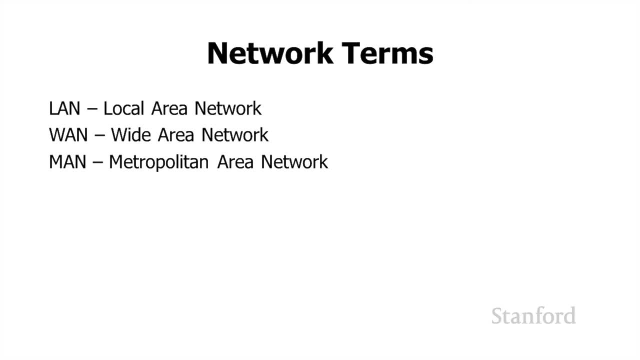 If you play computer games or you have friends that play computer games, you may hear them refer to a LAN party. This is a party where people bring their computers and get them networked together to play computer games. We used to do these back in the day. 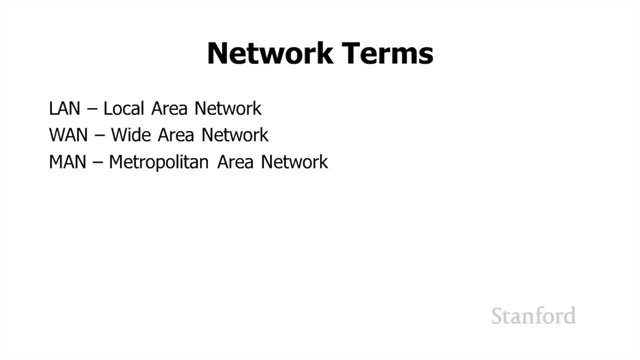 when Stanford changed its drinking policy at one point, We were trying to provide students with things to do other than drink, And so one of the activities the RCC started having LAN parties for campus. That was kind of cool. You may also hear about wide area networks. 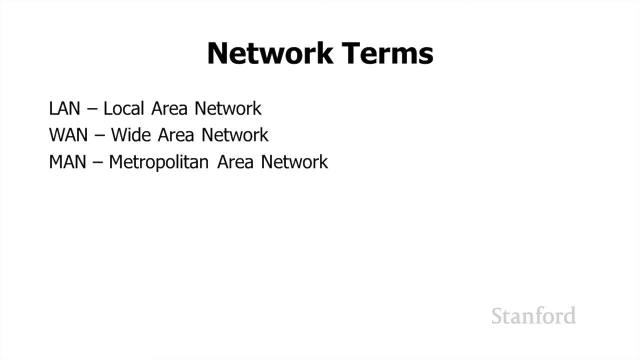 These are networks that connect Cities across continents or even across continents. You may also hear the term MAN Metropolitan Area Network. This is a network within a city, So if you have a friend that's saying I need to find a good man, they might. 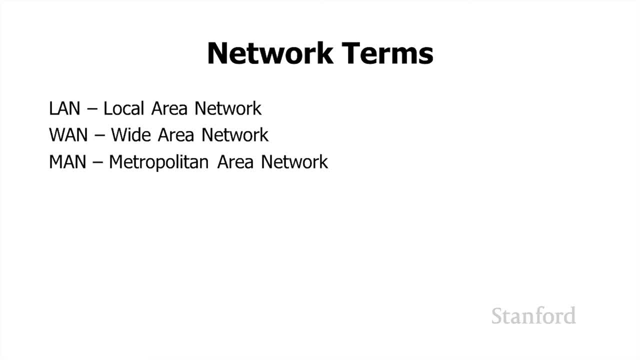 be referring to wanting to find a good guy, Or they might be thinking about which city they want to move to after graduation and making sure that that city has a good metropolitan area network. I'll have to admit, I've actually never seen MAN in this usage. 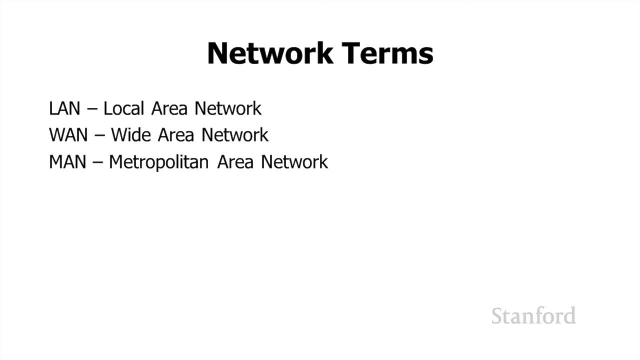 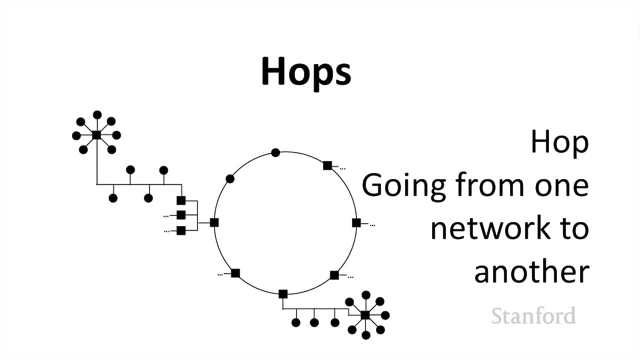 other than in network textbooks. But I'm fond of this joke, So you guys will have to put up with it. Another term you might run into is hops, As we talked about earlier. the internet is not a single network. It's actually a network of networks. 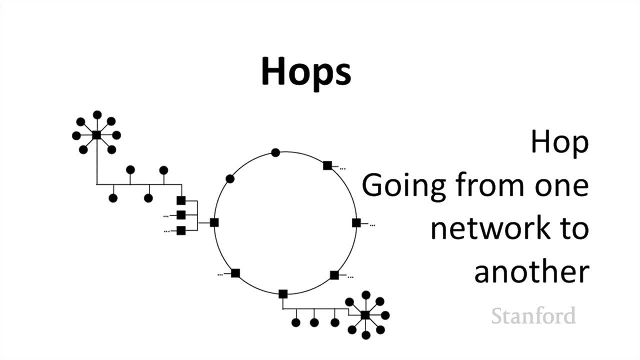 And so hops is referring to how many networks my message needs to go through in order to get to its destination. So if I'm trying to communicate with a friend, say, at Harvard, my message is going to have to go through many hops as it goes from the Stanford networks. 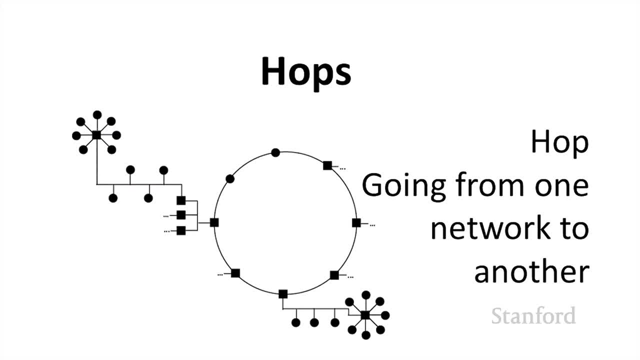 out to Stanford's connection with the wider internet. It goes through a bunch of internet backbone providers. It goes back out the other side. to get into the Harvard network It probably has to hop through a couple of different networks at Harvard. So these are all different things. 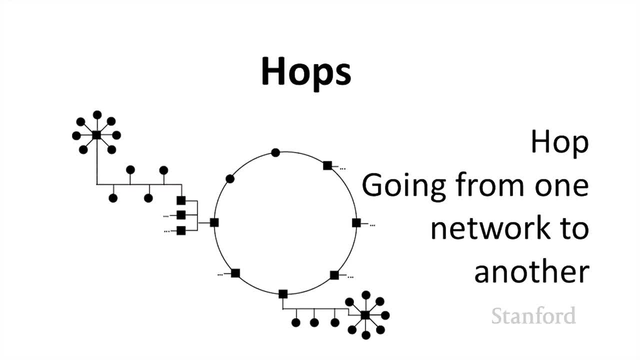 that the message has to do in order to get to its destination, And what's going to happen here is: there's a number of different things that's going to determine whether a message or data travels through the internet. One is going to be the connection medium. 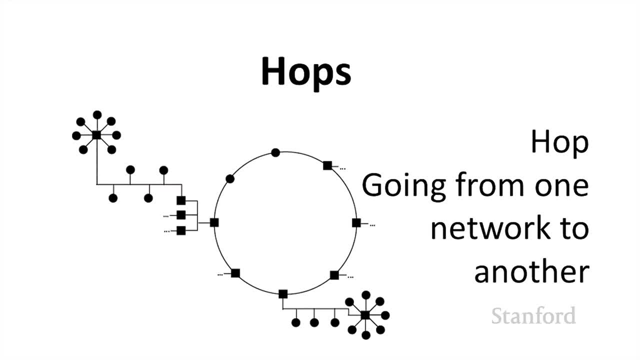 So if I've got fiber optic cable, that is going to be much faster than, say, plain old telephone service pods. But the other issue that's going to occur is every time message traffic goes from one network to the next network, there's also 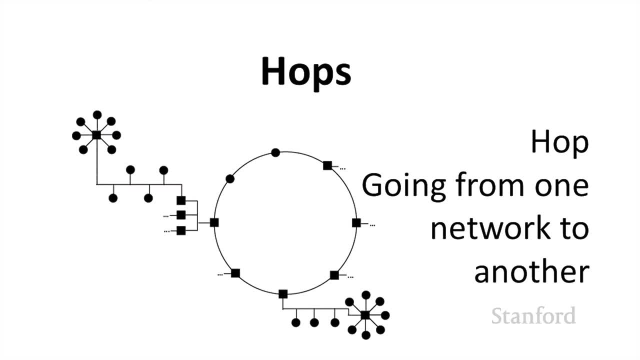 going to be a delay, because whatever we're using to connect those two networks together needs to spend some time looking at that message, figuring out: is this a message that's supposed to be going to someone on my network? Is this getting passed to another network? 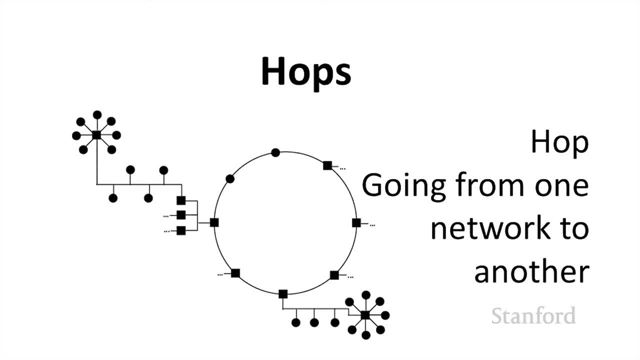 How does this need to get from this network to the other network, And so there's a delay because this actual processing has to take place. So the more hops we go through, the longer the message is going to take to get there. On a related note, you may hear people. 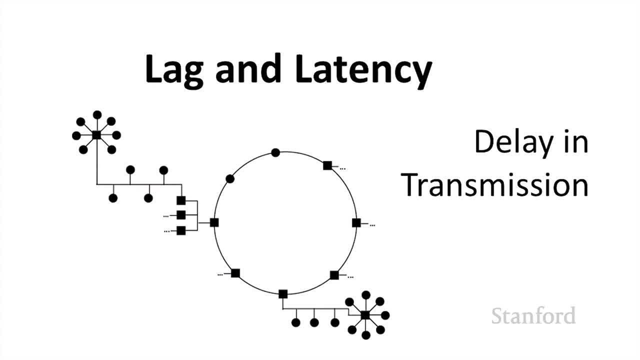 referring to lag and latency. Generally speaking, lag refers to the perception that the message is getting passed very slowly. For example, one of the things that I used to do as a resident fellow was when we were interviewing for new RAs. we would sometimes interview people. 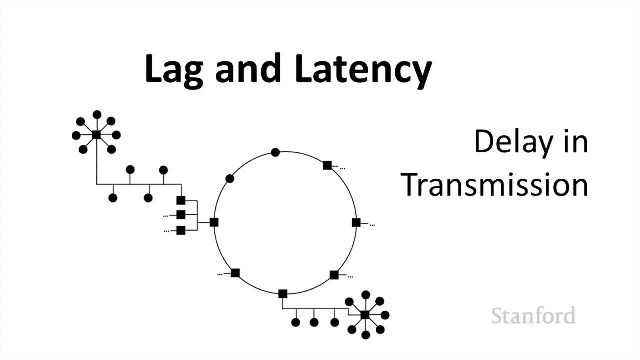 at various Stanford overseas, Bing overseas programs And you would notice, sometimes there would be a long lag between when someone spoke and when you actually heard their words, And so this is lag. This is the appearance that the network is not doing well. Another time you'll hear the term lag. 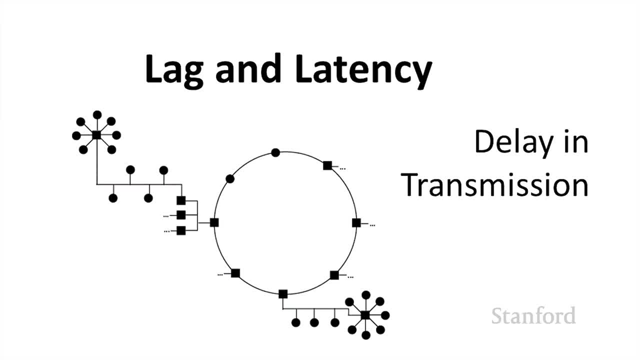 is: you have a friend who plays first person shooters and they're like: That wasn't my fault, It was the lag. Actually, it was their fault, They sucked. But the idea here is they tried to move their character in a particular direction. 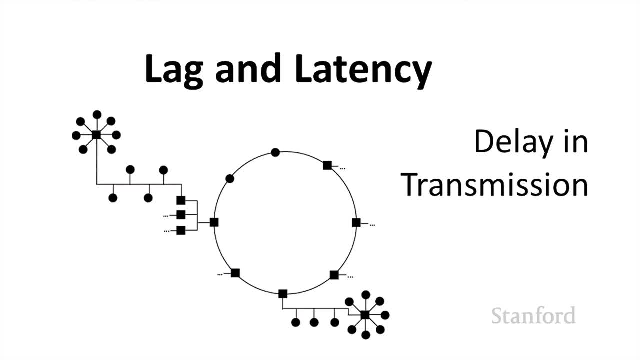 And because of the delay in network traffic they ended up getting shot. It wasn't because they didn't move quickly enough. It was because the message had to travel through too many slow connections or too many hops, or there was just too much. We'll talk about this in the next lecture. 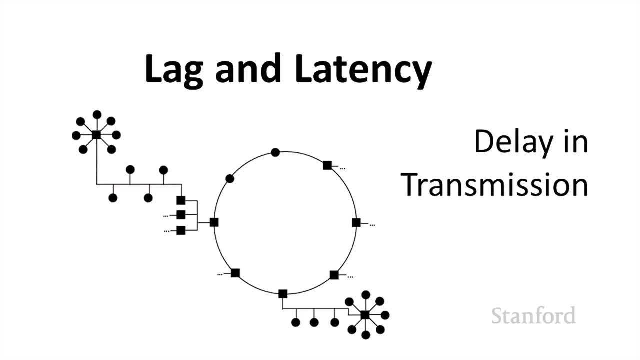 There was too many other packets traveling through the same network Anyway, so the end result was the information that they moved did not get to the server in time. The term latency generally is a slightly more technical term referring to the amount of delay involved in a transmission. 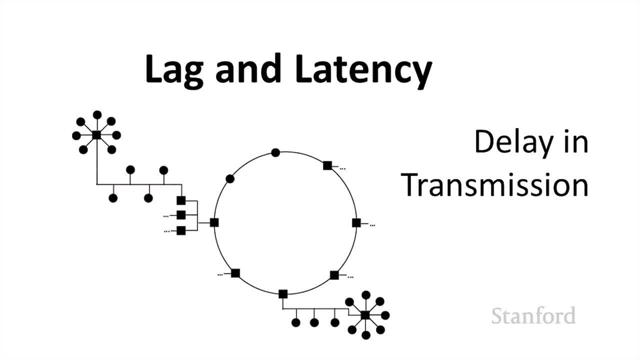 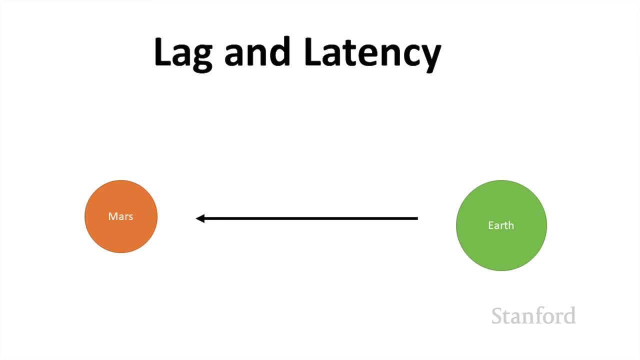 But these two are often used more or less synonymously. I should mention that lag and latency are not necessarily directly related to the speed of the connection, And so the idea here is: you could have a lot of bandwidth and you could still have lag and latency. 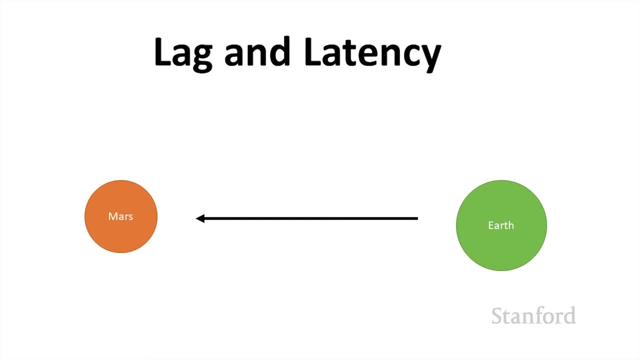 And so here's an example here. Suppose we are sending a message from Earth to a spaceship traveling around Mars. We've got several different things that we need to think about here. How much bandwidth do we have? Let's say I'm sending a new copy of the latest movie out. 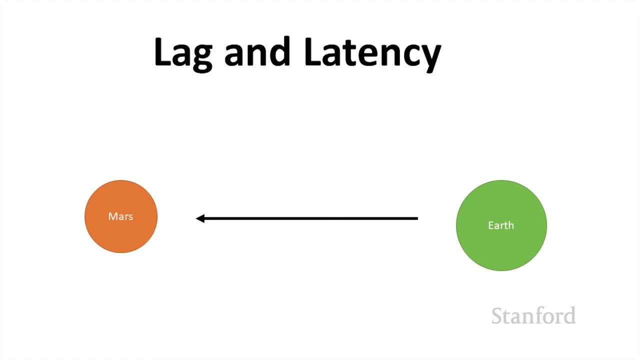 I don't know. I guess there aren't any movies out right now. But let's pretend Mulan is out And I've got an astronaut out there and she really loves Mulan. She loves the cartoon version of Mulan. 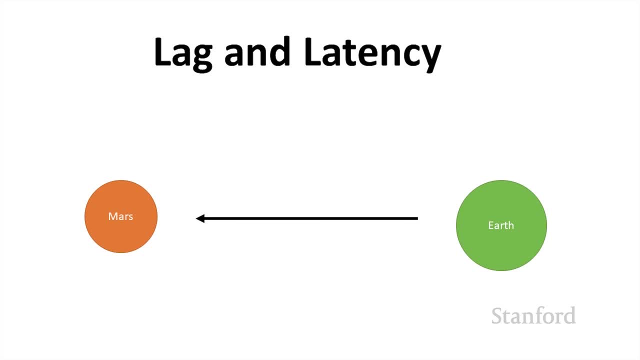 and the new live action version of Mulan is out And we want to send her a copy and she's out of Mars. So if we have slow bandwidth, it is going to take a long time for that entire movie to reach this destination, regardless of how far away. 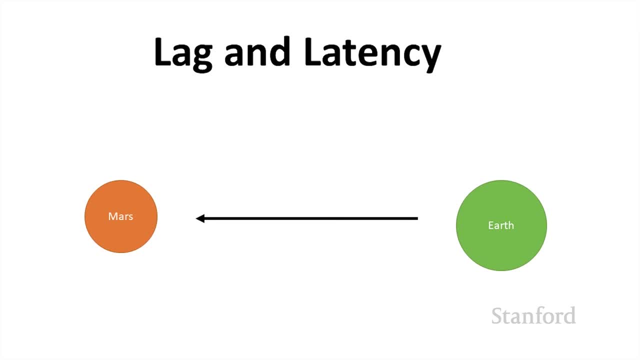 that person is. So let's say two of us are on the same network. There's no hops between us, but we're connected by a plane all the way to the telephone line. It's going to take a long time for that movie to transmit over that telephone line. 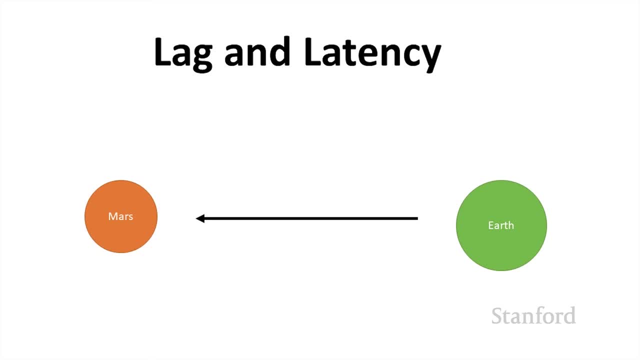 On the other hand, if we have a really fast connection because this person is really close to us, it's going to transfer very quickly. Now let's look at the situation where we're sending the data to Mars, Regardless of how much bandwidth we have. 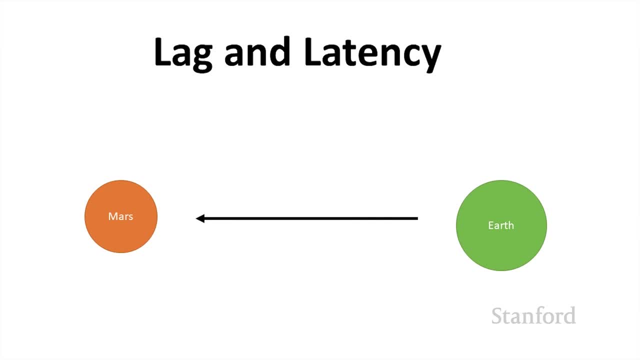 it is still going to take a very long time for those first bits to reach Mars. And if we have high bandwidth, once those first bits reach Mars the rest of the bits will fall very quickly. If we have low bandwidth, we still have the same delay, because it just 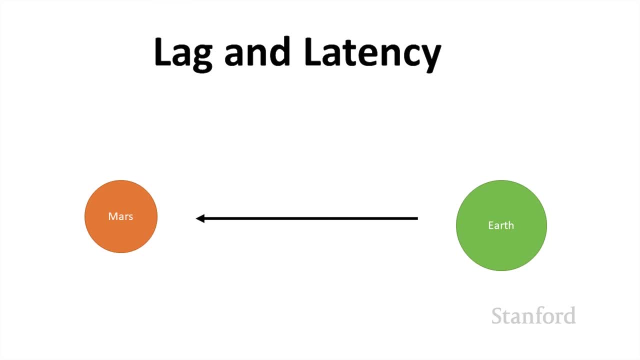 takes a certain amount of time for light to travel to Mars, But if we've got low bandwidth once those bits start reaching Mars, they're going to have to wait a long time between when the first bit hits there and when the last bit hits there. 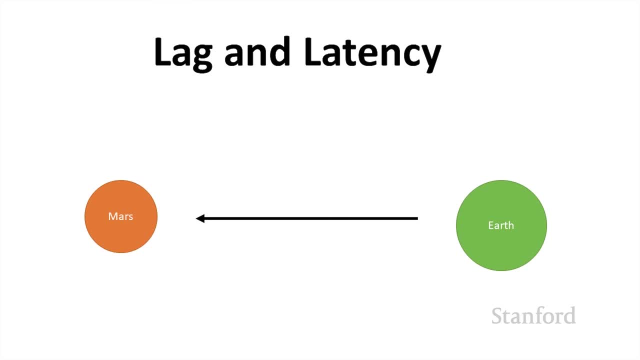 So the point of this is there's different issues involved here. It's not just a matter of, hey, I have a really high bandwidth connection or I have a really low bandwidth connection. Yes, those are important, But there's also a question of how far away is this person? 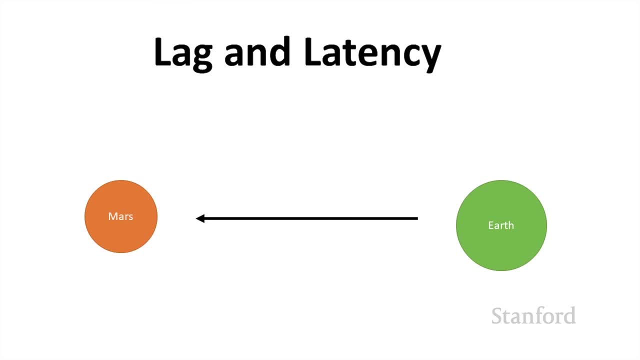 How many hops does this have to go through And things like that. And that's actually going to be an issue when you start worrying about things like web servers. We typically don't get into this, but since I've got a captive audience here, 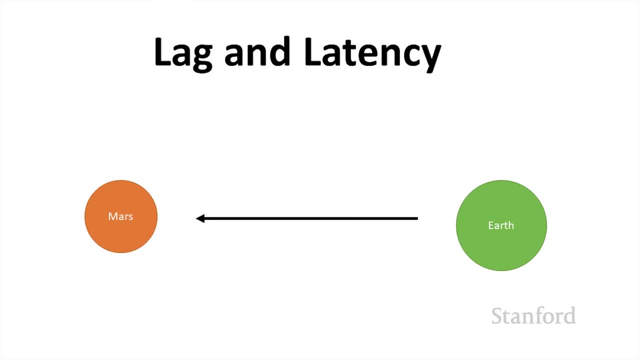 One of the issues that comes up is if I've got a web server and that web server is, say, in California and my customer is in Australia, there's a pretty long delay where the message needs to get transferred from my server here in California. 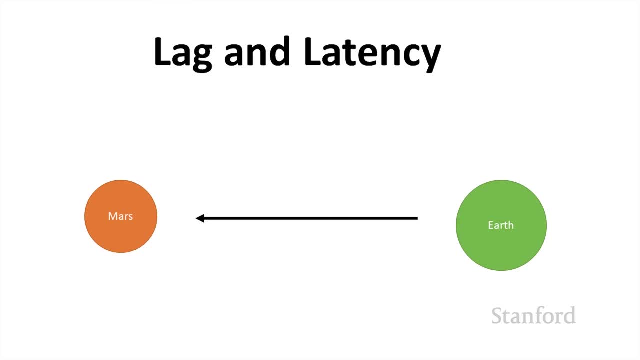 through a whole bunch of hops to get to Australia, And so a better way to handle this is to use something called a content delivery network, or CDN, And what a CDN does is it takes the files that would normally be in my server here in California. 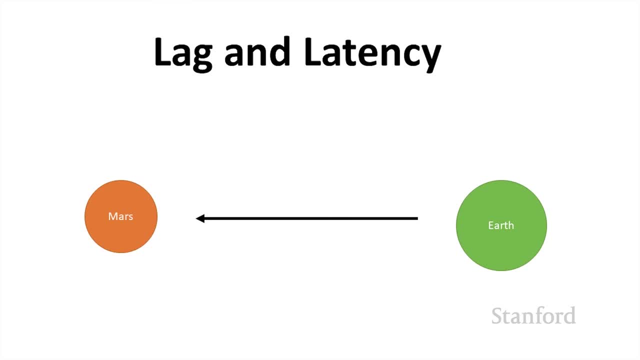 and it distributes to a whole bunch of different servers around the world. So there will be a server in Australia or Oceania, There will be a server in, say, Asia, There will be a server in Europe And there will be a server in the United States. 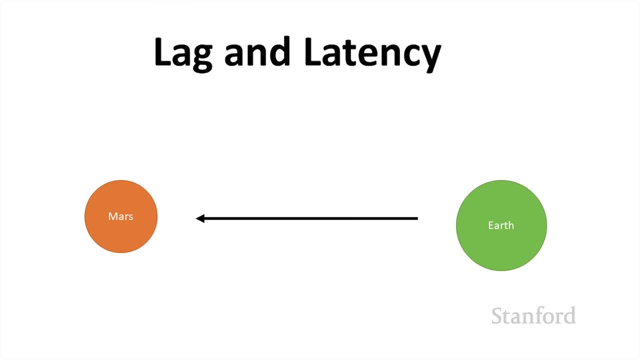 There will be a server in Africa, And wherever the person is trying to access our information from, they will get it from the nearest server, And so there will be fewer hops to get to that server. There will be less lag. There will be less latency. 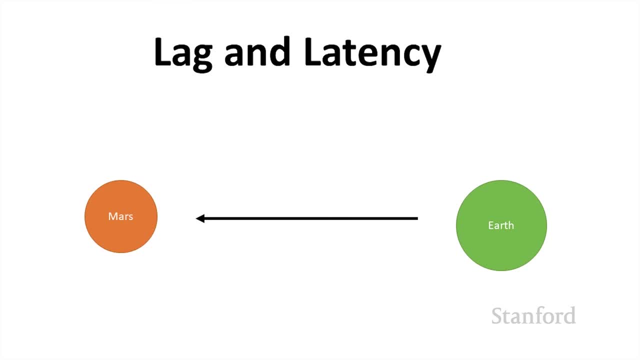 And the information will get to them much faster. So if you're going to come up with a server and you think that you're going to have a global audience, contracting out to a content delivery network might be a great idea. All right, so that's it for now. 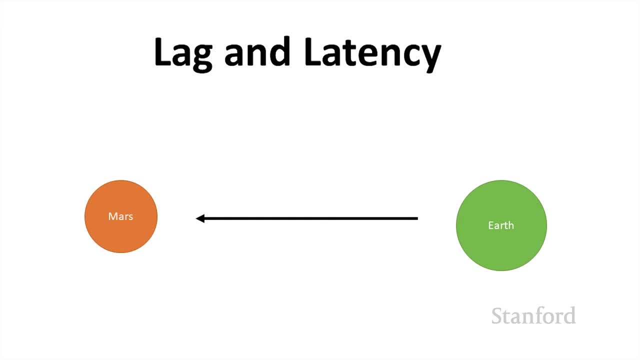 In the next lecture we're going to talk about how to identify individual computers on the network, And the next lecture on Friday we're going to take a look at different protocols that are used governing how information travels through the internet. I'll see you again soon. Bye. 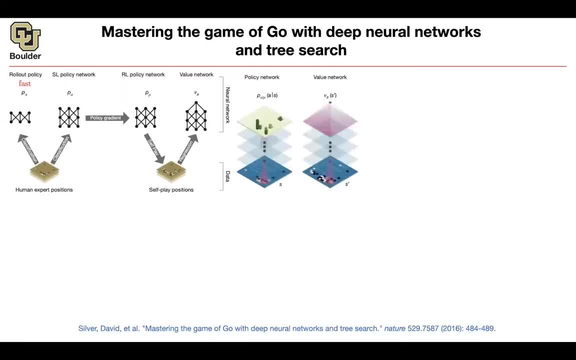 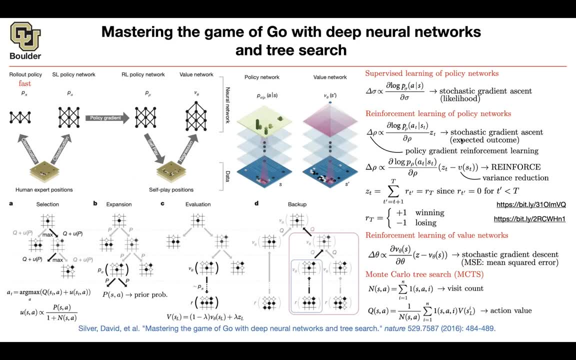 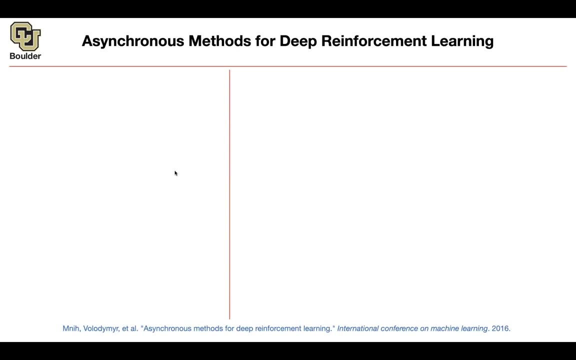 Let's move on This paper we covered, so I'm not going to go into the details anymore, but this is an overview of what we covered last session And this was the policy gradient. So you were doing reinforce- Let's move to asynchronous methods for deep reinforcement: learning What is?